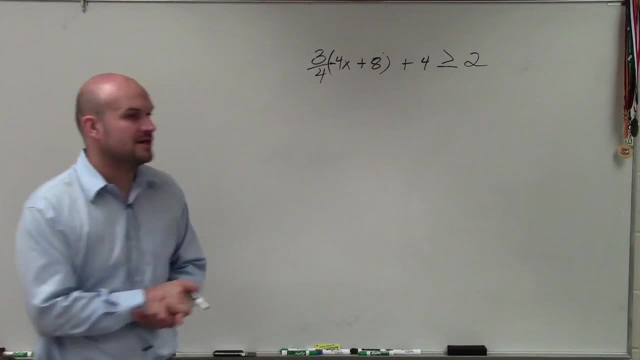 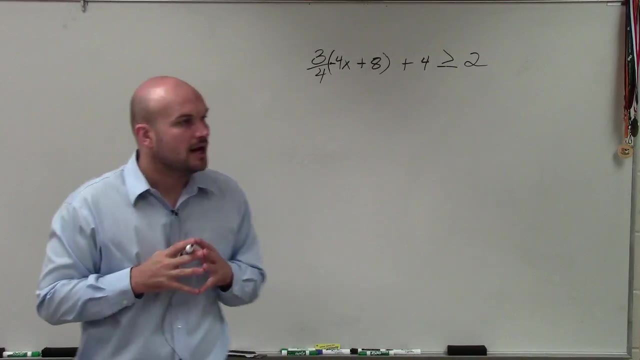 but yes, this would be the exact same one. okay, So in Jasmine, when we're going through this one, there's actually going to be two different ways. I want you guys to go through this problem. all right, We can go ahead and apply with fractions, or we can obviously just always. 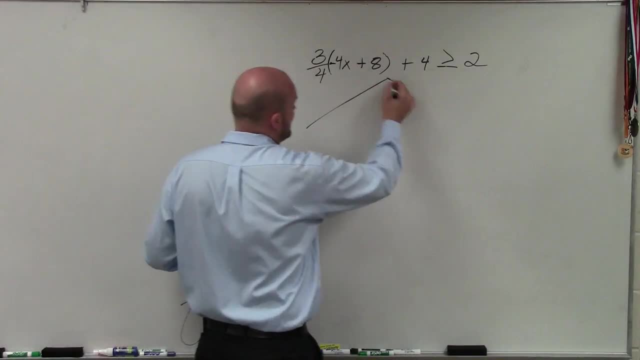 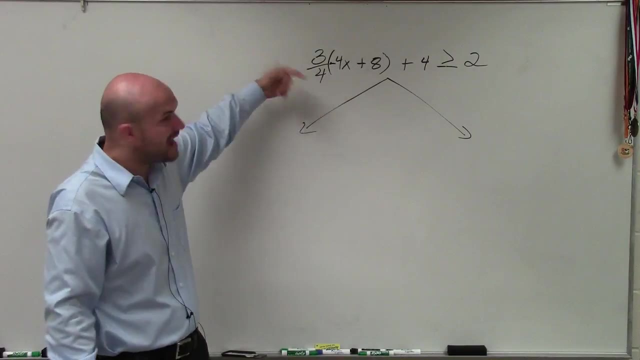 get rid of fractions, And we went through this a couple times before. The first thing, guys, whenever you see a fraction is the first thing I would say is: just get rid of your fraction. right, We have a fraction because 4 does not divide evenly into 3.. So to undo 4 dividing 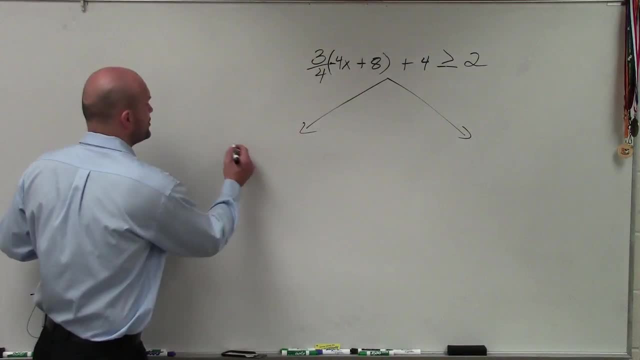 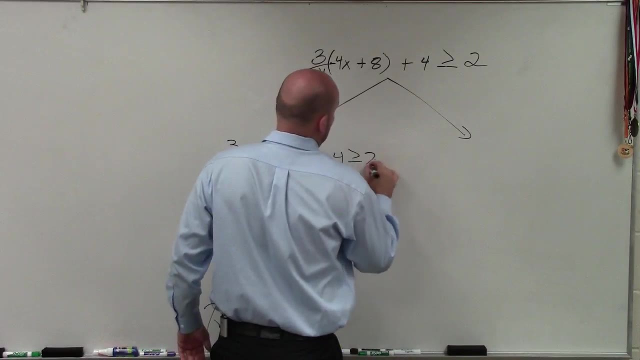 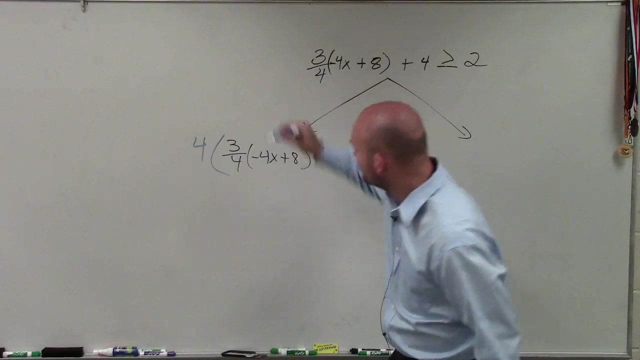 evenly into 3 is undo dividing by 4, which would be to simply just multiply By 4.. So just because I'm writing this up here, I'm going to take everything and multiply it by 4.. So you multiply the 4 times here. you multiply the 4 times here. 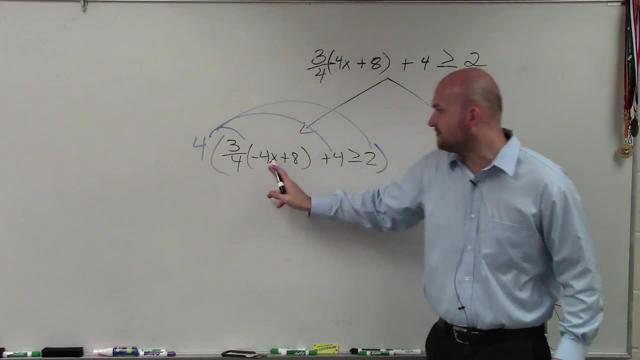 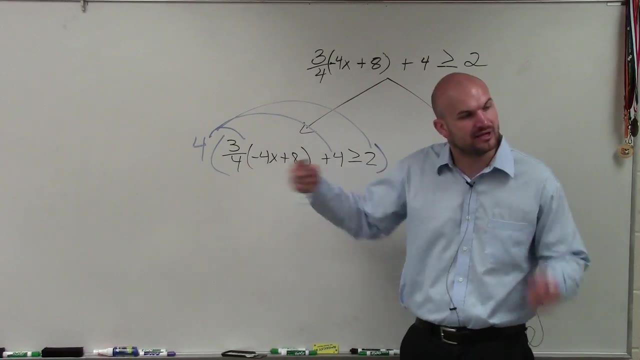 and the 4 times here. The reason why I don't multiply the 4 times this is because 3 fourths times negative, 4x plus 8, that is considered one term together, because they're connected by multiplication. They're connected by multiplication. 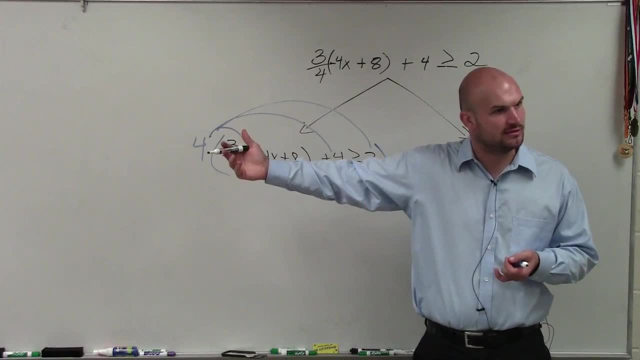 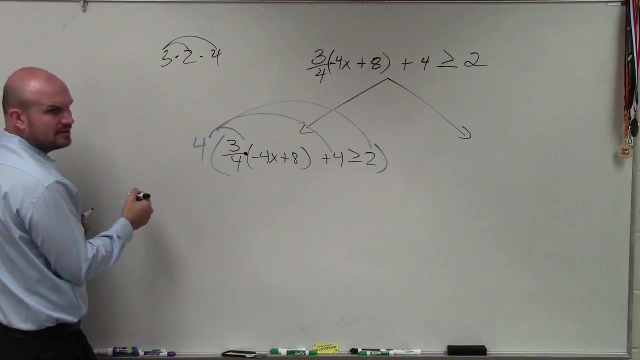 right here. So you don't distribute across multiplication, right? When I say 3 times 2 times 4,, you don't say 3 times 2,, 3 times 4,, right? No, 3 times 2 times 4 is 3 times 2. 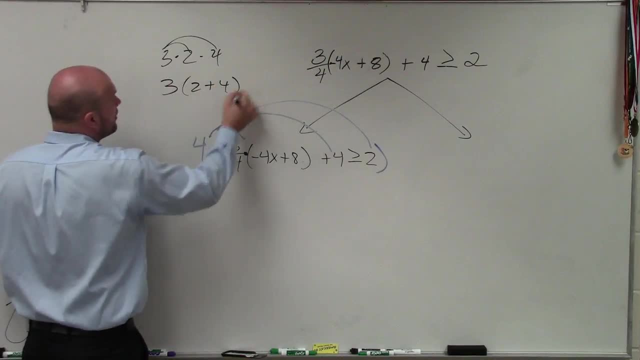 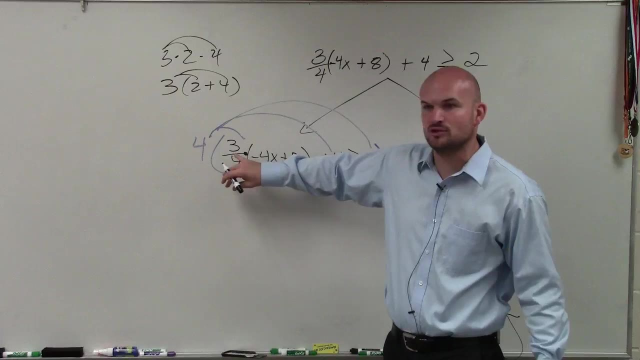 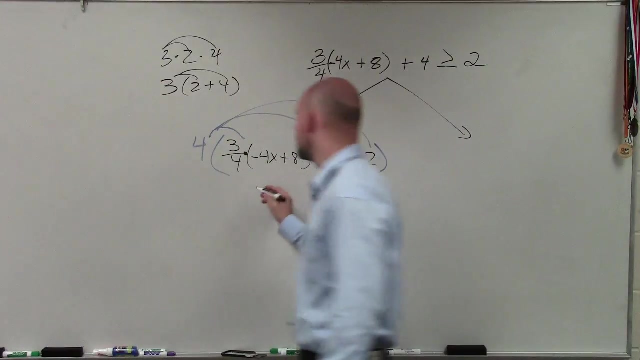 times 4.. If it was 3 times 2 plus 4, then yes, you distribute across addition, across subtraction, But we don't distribute across multiplication. Does everybody understand that? Because it's a confusing point here: 3 fourths is just going to be 3 times negative, 4x plus 8.. 4 times 4 is 16.. 4 times 2 is 8.. 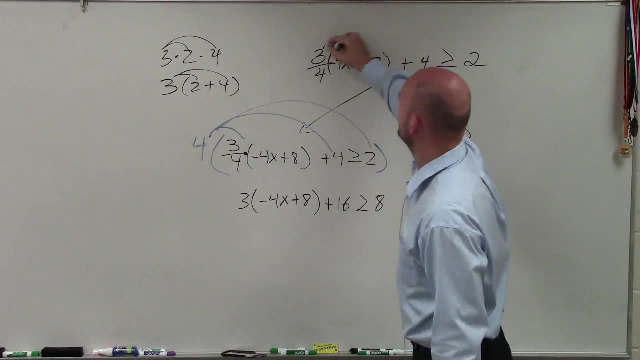 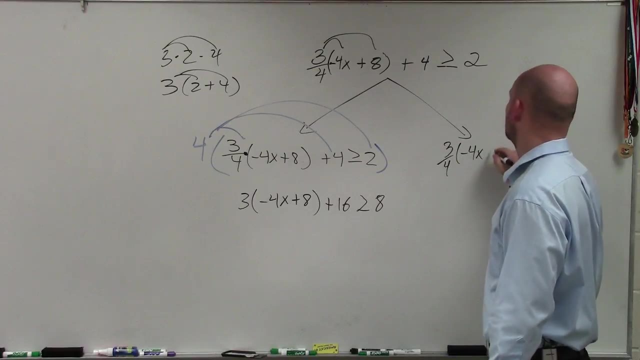 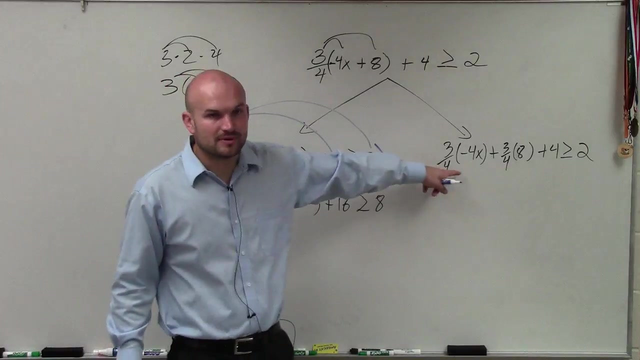 The other way you could do this is simply just apply distributive property. So I could do 3 fourths times negative 4x plus 3 fourths times 8. Plus 4 is greater than or equal to 2. So you could also just apply distributive property. 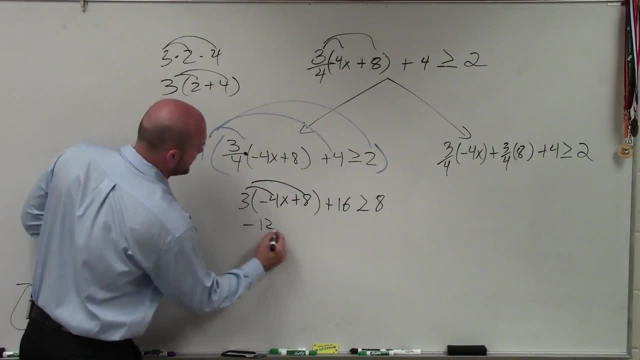 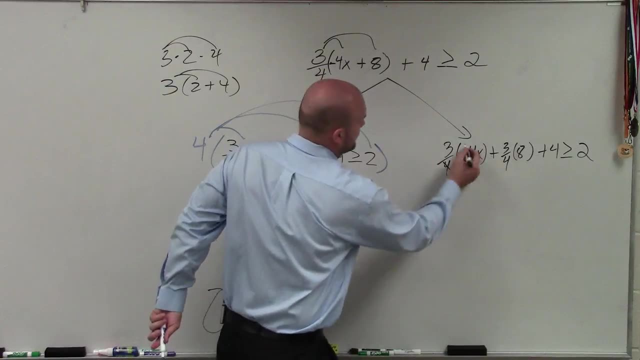 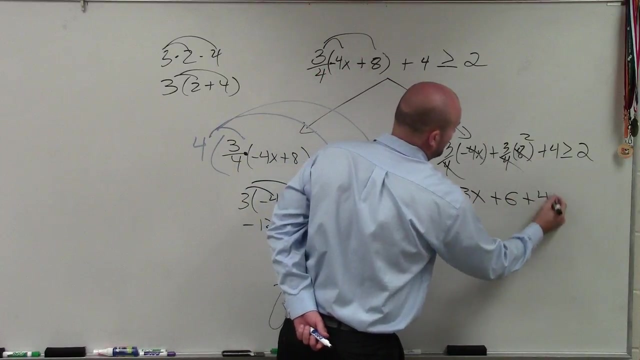 Now let's work through this. If we apply distributive property here, you guys would probably like that Negative 12x plus 24 plus 16 is greater than or equal to 8.. Over here the 4s divide out. I'm left with negative 3x. Here those divide into 2.. 2 times 3 is positive 6. Plus. 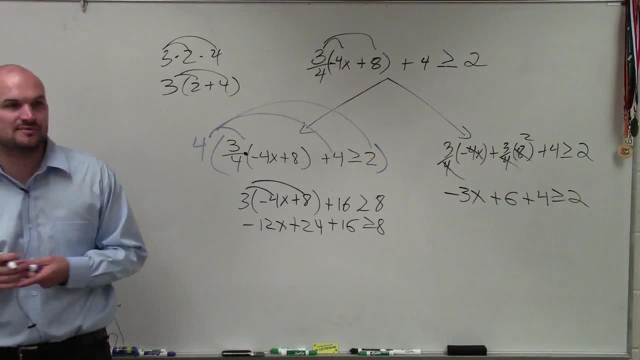 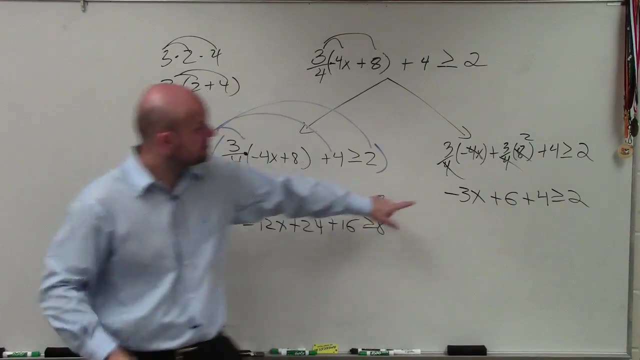 4 is greater than or equal to 2.. Anybody have any questions on what I have done, Because I'm doing the problem twice. Yes, Well, how did you get 3? Here? No, But how did you get 3 over here? 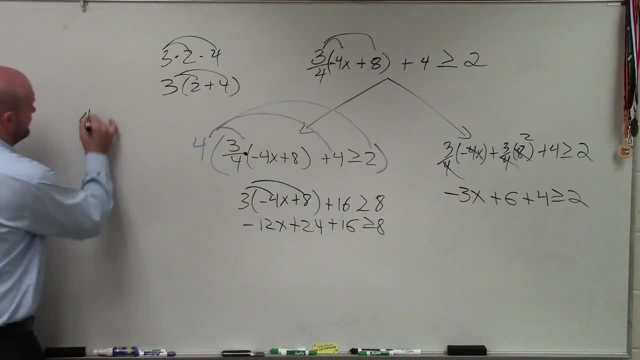 Here Yeah, When I multiply 4.. 4 times 3: fourths. But how about we cancel out? Well, you could think about them canceling out. They're not really canceling out. 4 times 3 is 12. divided by 4 is equal to 3.. Or 3 over 1, which equals 3.. 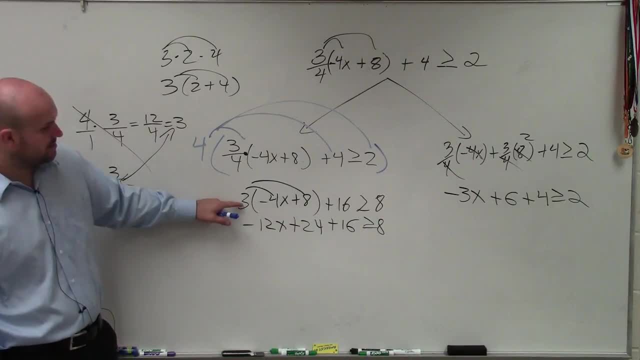 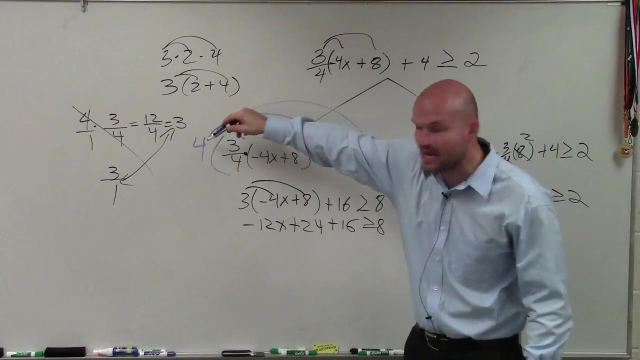 Same thing, But yeah, that's all I got 3.. Right there, The 4.. Does that make sense? You're multiplying 3 times 4 times 3 fourths. So yes, you could say the 4 is divided into 1, which just leaves you with the 3.. 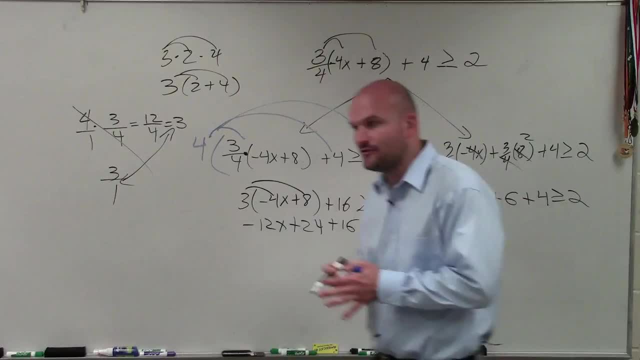 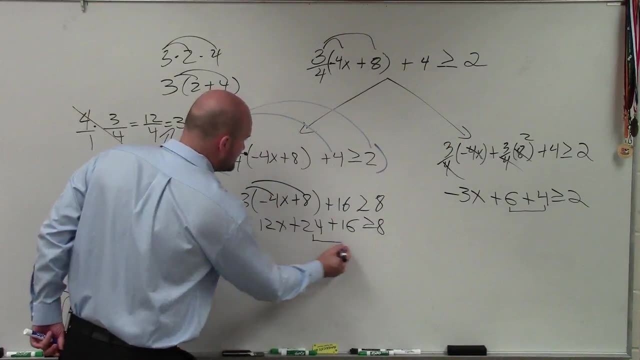 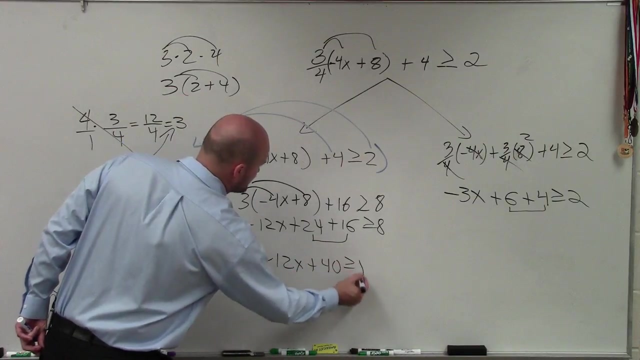 Now the next step is again, before we get to this, we've got to make sure that we combine our like terms. You guys see, we have these two terms right here and these two terms right here. So I have negative 12x. This becomes 30,, which is plus 40,, is greater than or equal to 8.. 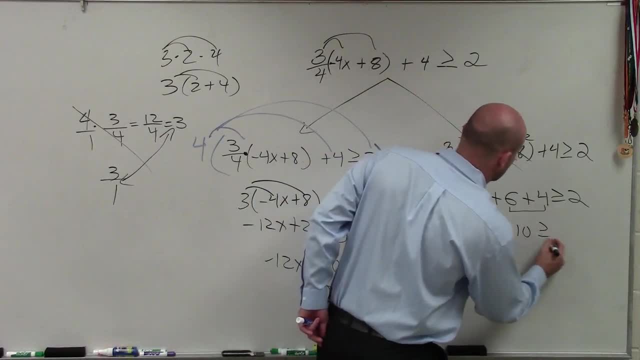 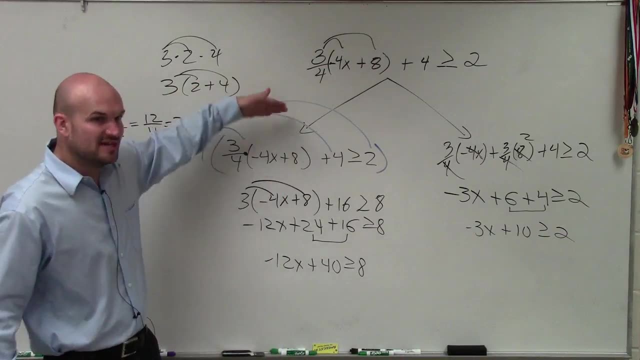 Over here. I could say: negative 3x plus 10 is greater than or equal to 2.. Now I have simplified it down to a two-step equation. Now again, guys, I know I'm doing it twice. This obviously is. they're not exactly the same, but you'll be able to see we'll. 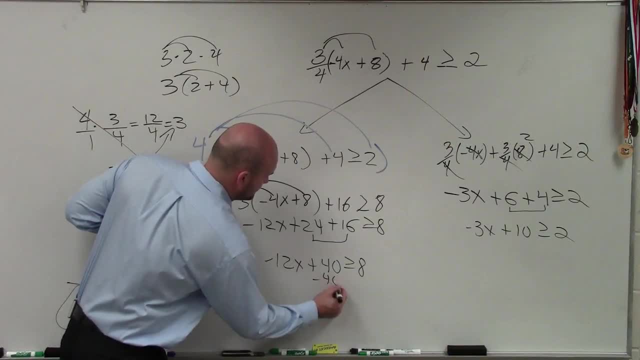 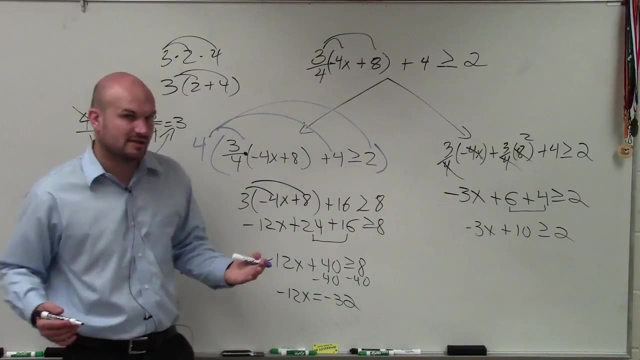 get the same answer. So I subtract 40. Subtract 40. Negative 12x equals a negative 32.. And the important thing that I wanted to have you guys get with is now I'm dividing by a negative 12.. 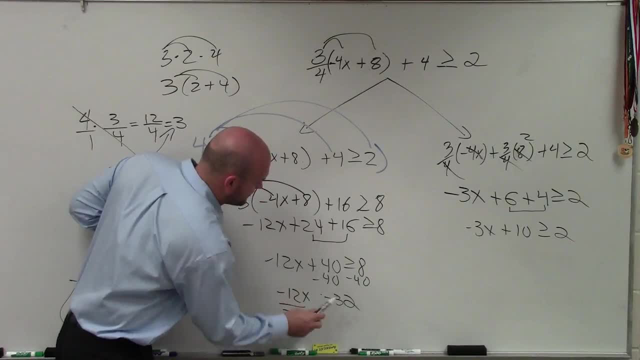 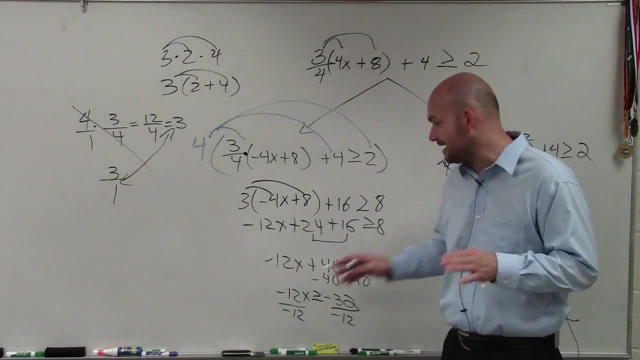 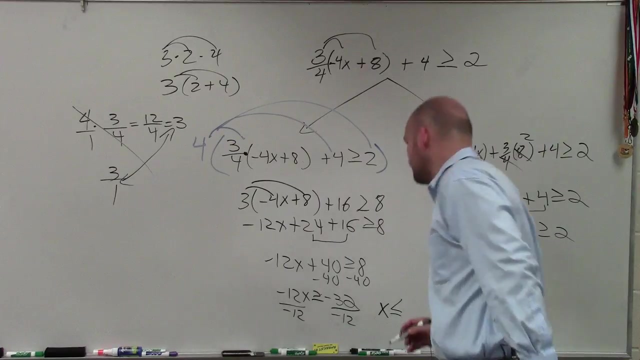 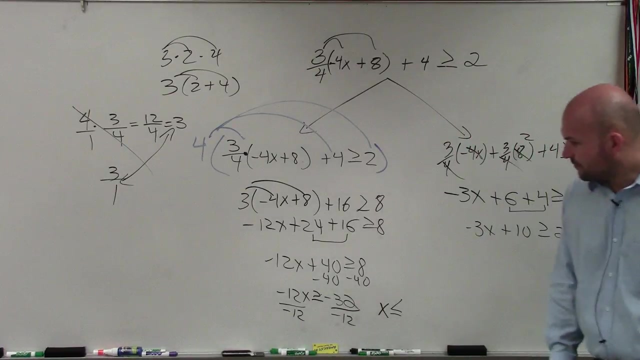 Ah, shoot, What happened? So when I divide by a negative 12, though I got to make sure- whenever you multiply, divide by a negative number, you have to flip the sign. So I have: x is now less than or equal to 32. divided by 12 is going to be 1,, 2,, 24,. 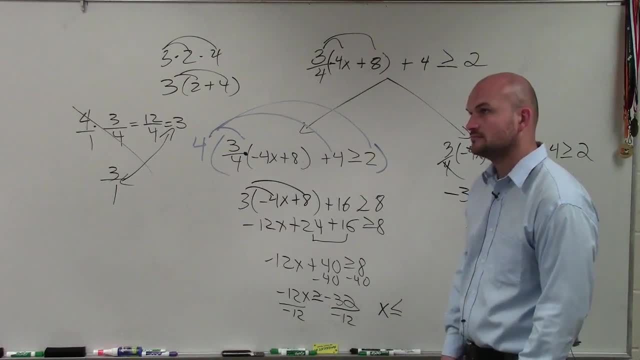 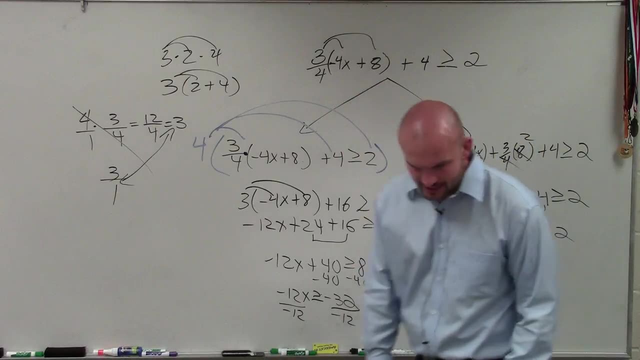 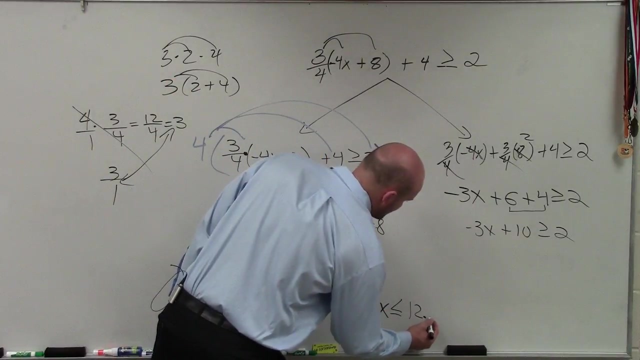 and 8 twelfths. Right 24, yes, and 8 twelfths. 8 twelfths reduces down to 4 sixths, which is 2 thirds. So I'm just going to estimate with the decimal. You guys do not have many decimal. 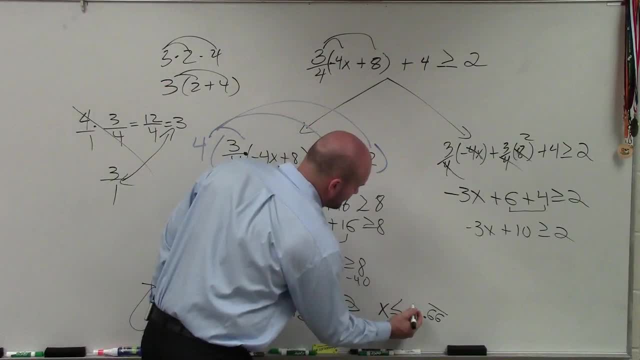 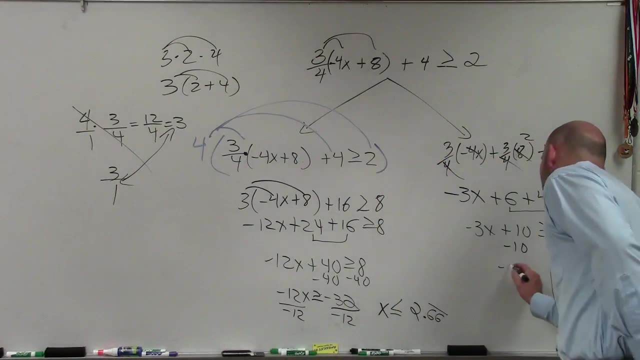 2.6.. 2.6,, yeah, 2.66.. And we can go and verify that over here too. If I subtract 10, subtract 10, negative 3x is greater than or equal to negative 8.. You guys can see that, Yeah, how. 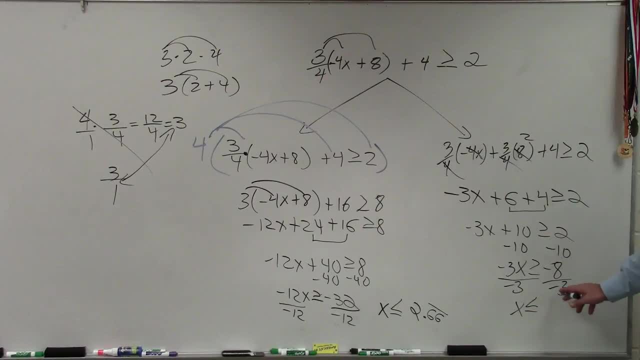 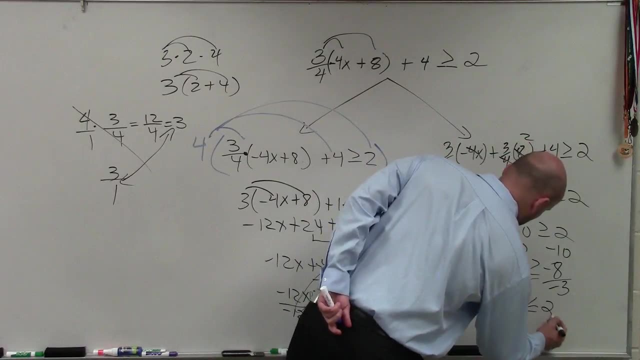 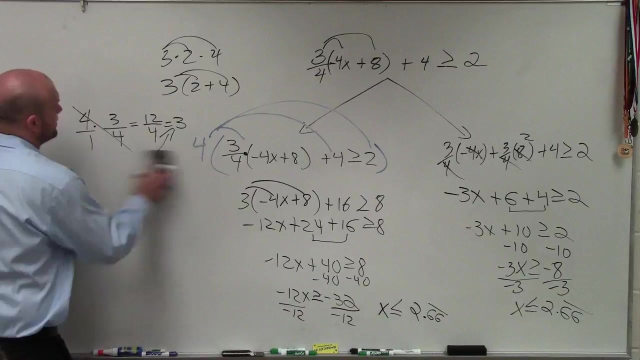 many times does negative 8 go into there? I'm sorry, negative 3 going to negative 8.. It goes in there two times, with 2 over 3 remaining, So you're not going to have many fractions, but let's just go through again what to do with this. 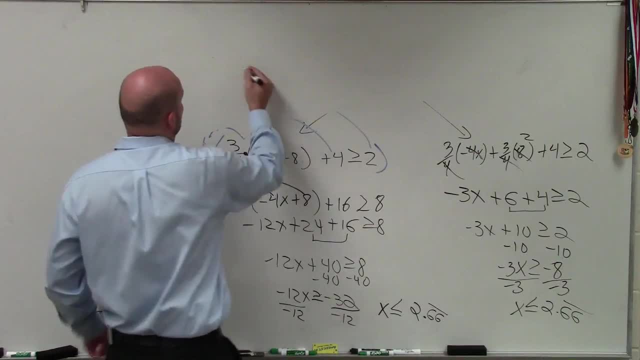 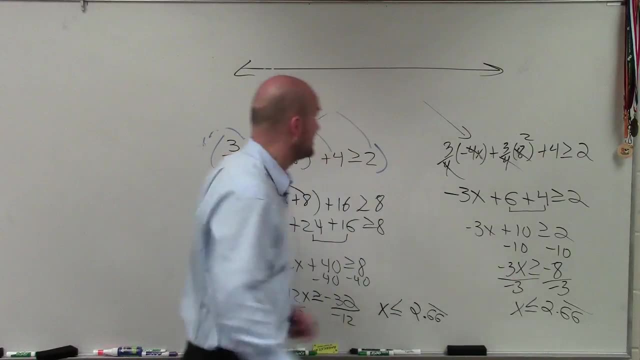 And sorry I had to make up the problem. Ah, you guys are running out of time, All right. so just please note, guys: whenever you multiply, divide, you flip the sign. Now we're dealing at 2.6, so I can say, all right. 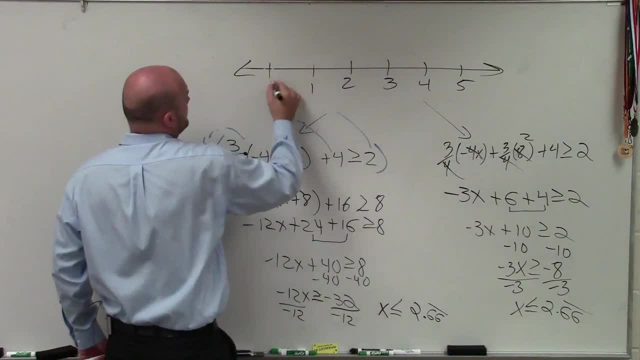 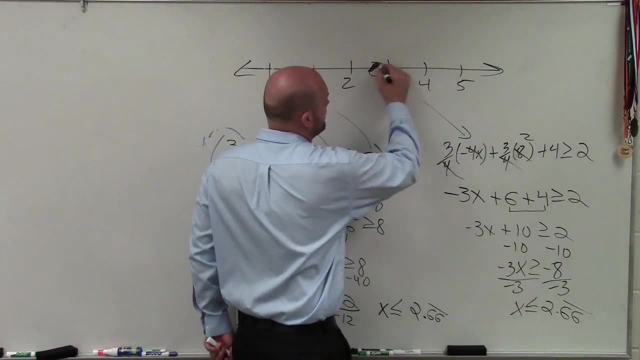 there's 2, there's 3,, 4, 5, 1, 0.. 2.66 is going to be roughly right there. Notice that it's less than or equal to, not less than, So it's going to be a part of my solution. 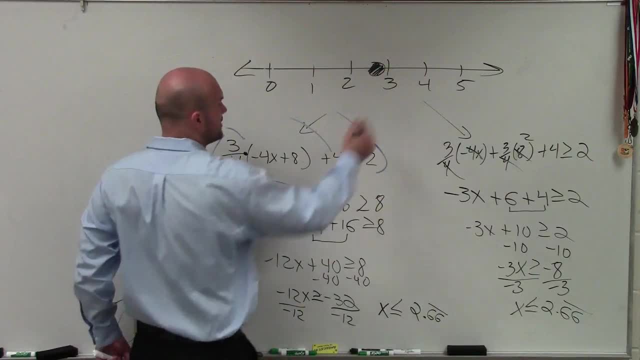 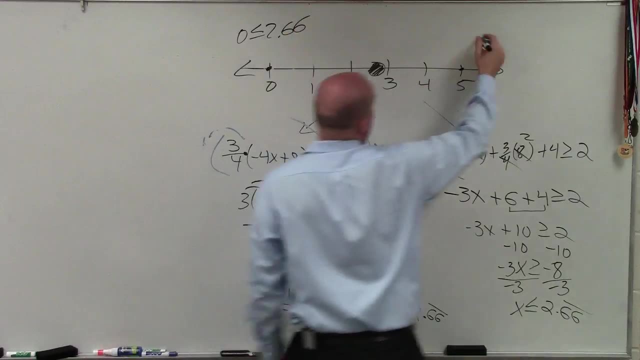 And if you're having trouble determining should I go left or should I go right, just what I do is pick points to the left and to the right and then plug them in. Is 0 less than or equal to 2.66?? 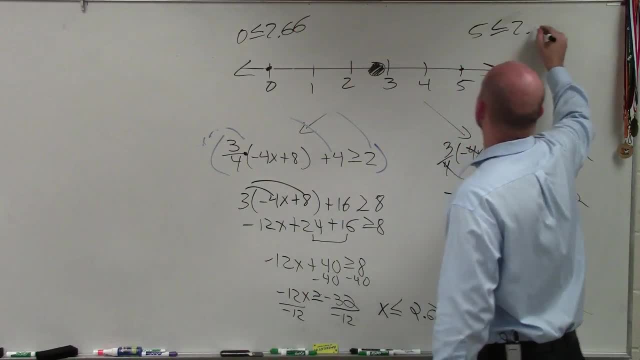 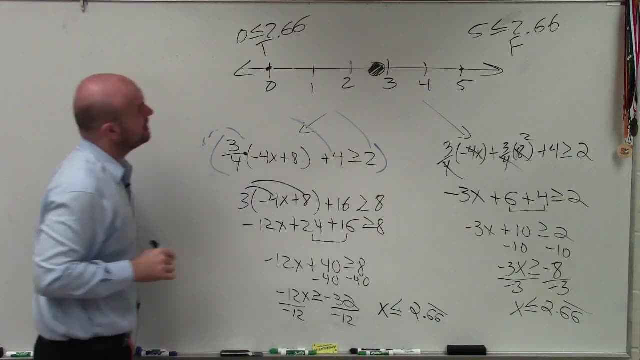 Is 5 less than or equal to 2.66?? Obviously, 5 is not less than or equal to that. That's false. Obviously, 0 is less than 2.66, so that's true. You always shade towards true, away from false. 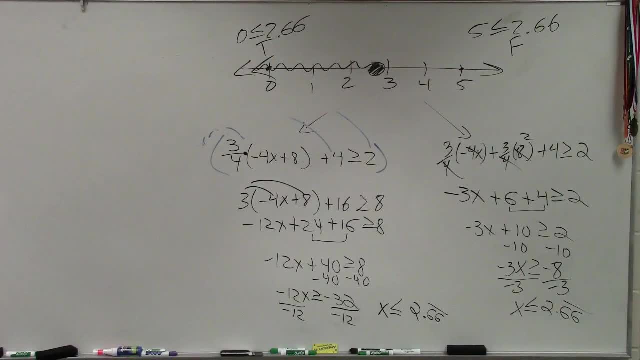 And there you go. So it's OK to have decimals. ladies and gentlemen, There are a couple problems on your homework that you do have decimals.